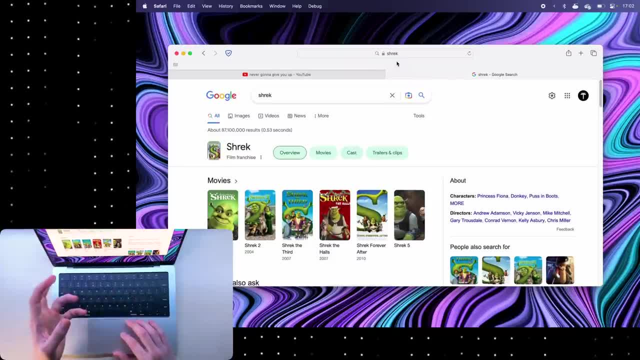 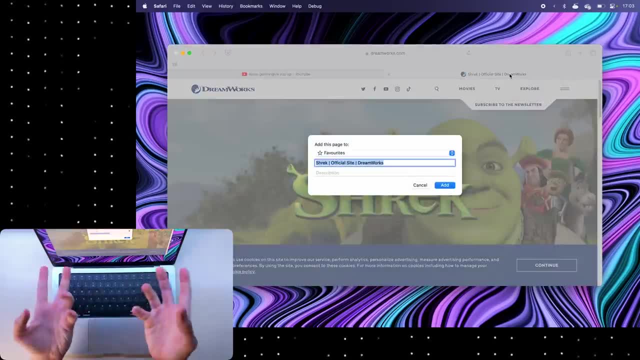 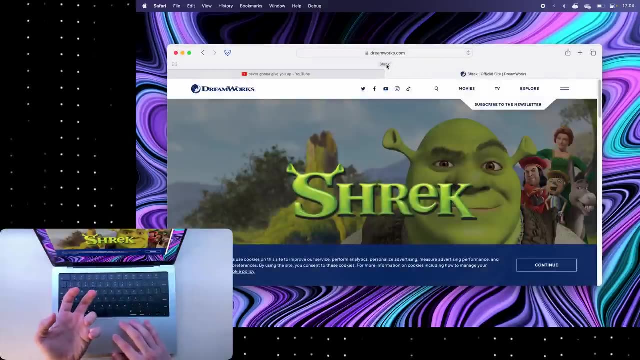 shift B to toggle the hiding or showing of the bookmark bar. And I don't have any bookmarks right now, so if I want to add one, I would click command D and I can add this to my bookmarks, which in Safari, for some reason, is called favorites. Anyway, I can click add and now it will show up. 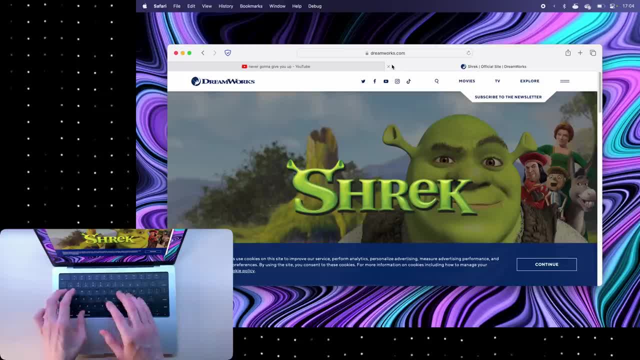 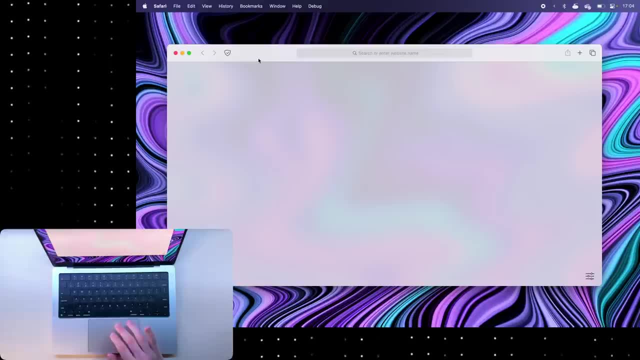 here. If I want to hide bookmarks again, command shift B and command shift B to open them again. Next, you'll notice that the top of my Safari probably doesn't look the same as yours, and that's because you can right click up here and click customize bookmarks. 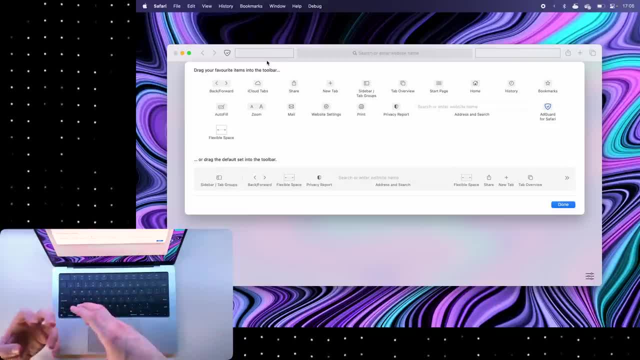 Toolbar here you can basically drag everything out that you don't need like. so just drag, put something in here. if you need something, What I have here is basically just a new tab page. Then this one brings up that mission control that I talked about before, and then the back and forward. 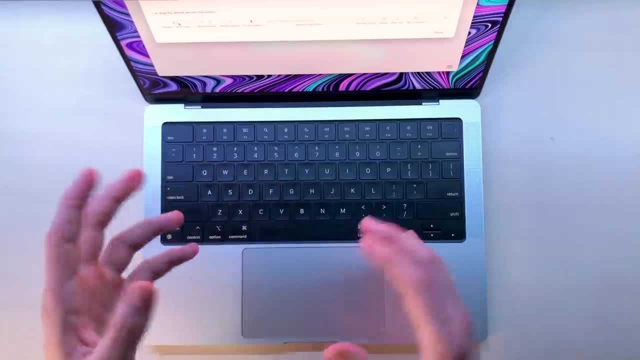 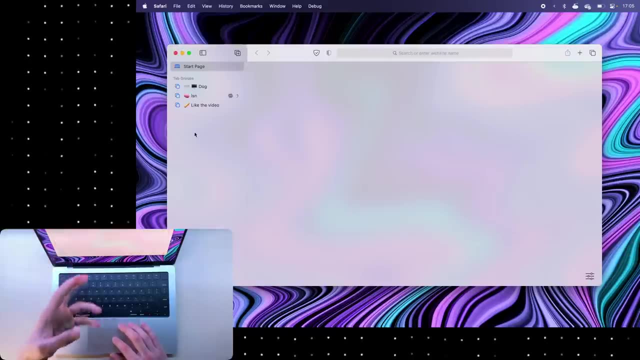 buttons here. This is an extension which I'll talk about later. Also, if you don't want to remember the shortcut command shift L to open your tab groups, you can add this one right here and then, if I click it, it will open up my tab groups. 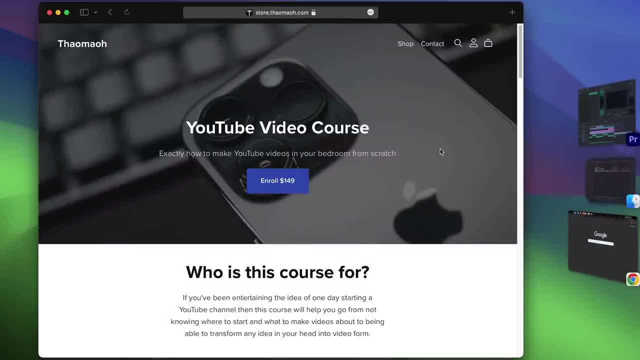 If you ever had a thought about starting a YouTube channel, I recently released my YouTube video course where I'll teach you about how to make faceless videos in Premiere Pro in something like five hours. So you know. link in the description Now, if you want to change things like your. 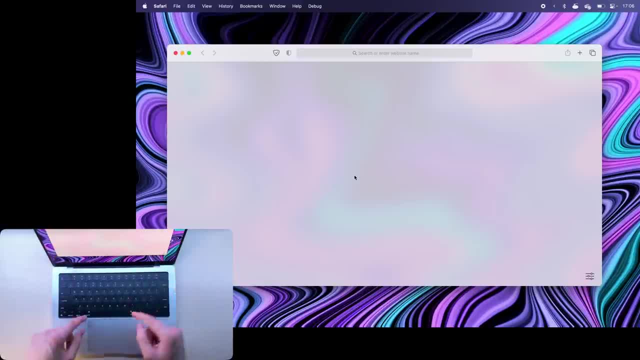 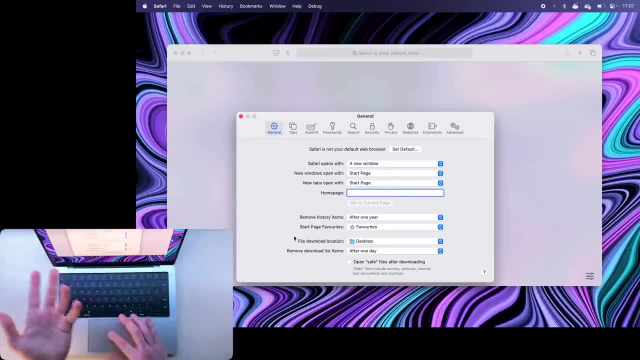 home page address or your default search engine. you can again go to settings, command comma, and then under search you can pick your search engine. Now for the home page. you can go into general and set up your default home page here so that it immediately opens your. 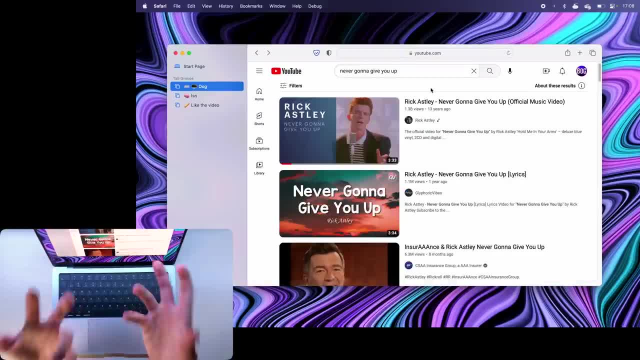 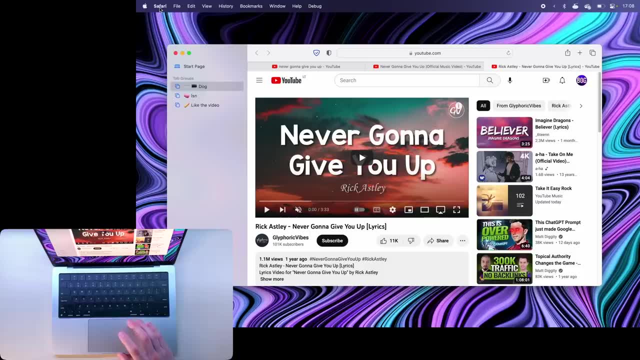 favorite song as soon as you launch Safari every time. Now, if you want YouTube to stop autoplaying things when you open them in a new tab like this, What is this ad? You can click on Safari here and then go to settings for YouTube and then, under autoplay, select never autoplay and 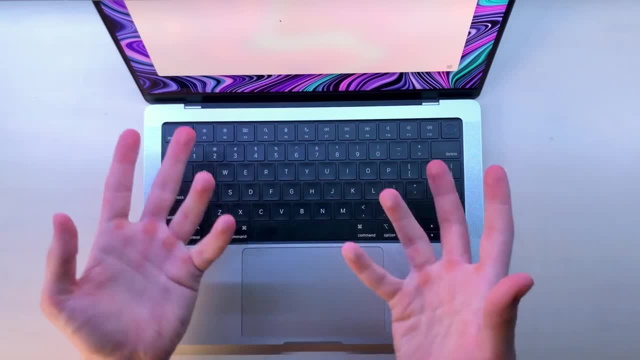 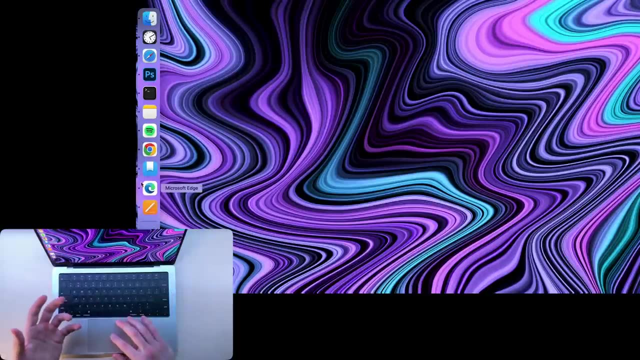 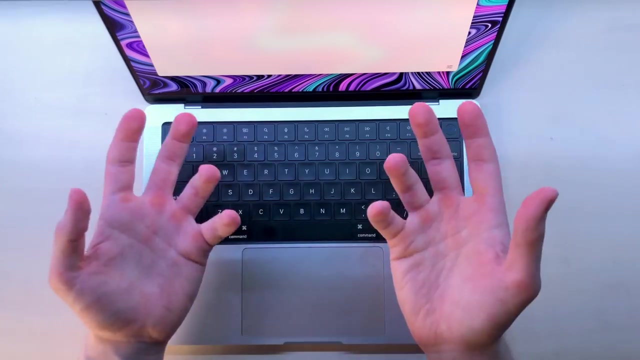 you can do this with any website. Now, unfortunately, Safari isn't the best PDF viewer that Mac has. I don't really like the default preview app either, So what I choose to do instead is just use Microsoft Edge, because it's, frankly, a great PDF viewer. Another thing that makes browsers cool is extensions.